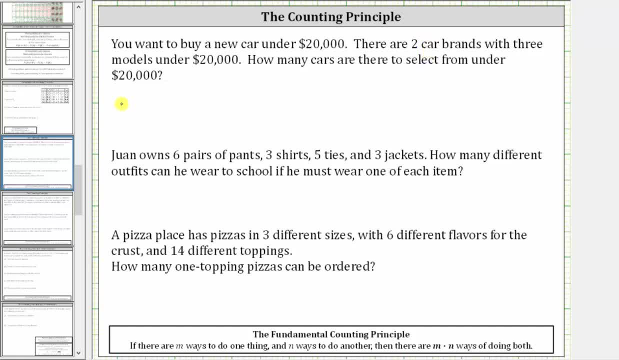 for the number of car choices. So you first must choose the brand, So let's call it brand one or brand two. Once you select the brand, you must select the model, and there are three models to select from. So under brand one, there are three models to select from. 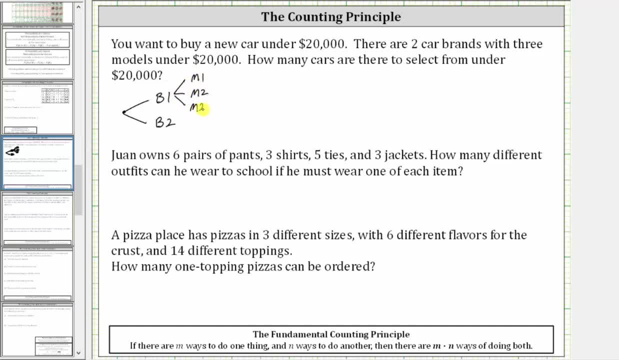 We'll call it model one, model two and model three. Under brand two, there are also three models to select from. Again, we'll call it model one, model two and model three. And now we can see there's a total of one, two, three. 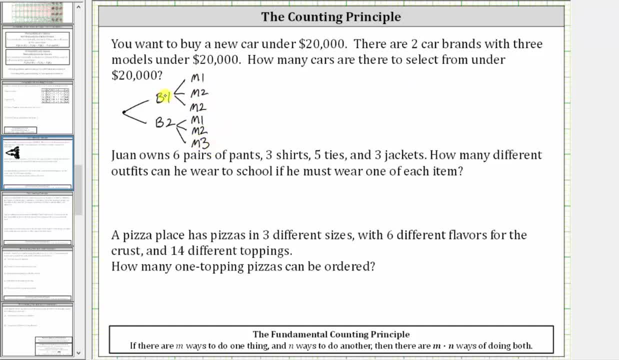 four, five, six cars to select from under $20,000.. So the answer is six cars. Which leads us to the next question, Which leads us to the fundamental counting principle, which states: if there are m ways to do one thing and n ways to do another, 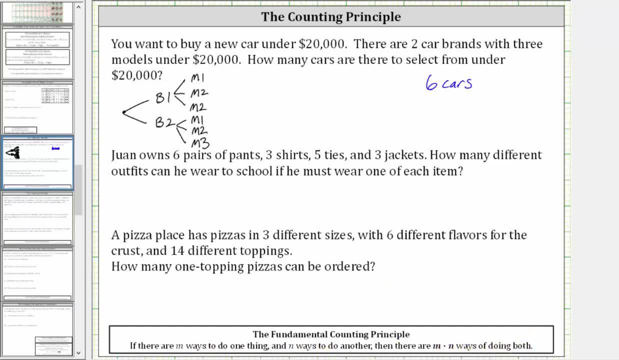 then there are m times n ways of doing both. So in our case, you must select the brand and then select the model, And since there are two ways to select the brand and three ways to select the model, two times three is equal to six. 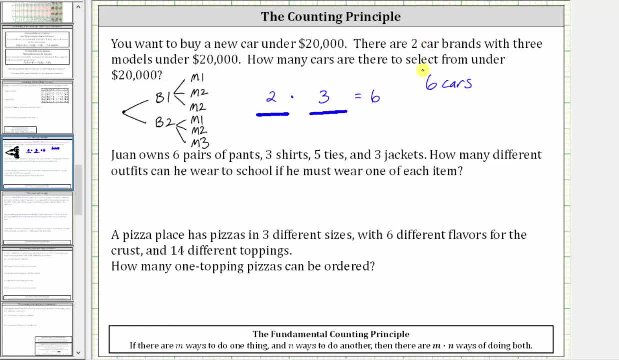 giving us a total of six cars to select from under $20,000. Again, where the first choice was the brand and the second choice was the model. For the remaining examples we will use the fundamental counting principle. So next, we're told, Juan owns six pairs of pants. 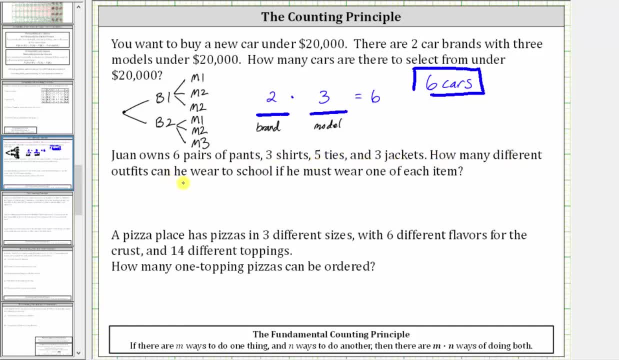 three shirts, five ties and three jackets. How many different outfits can he wear to school if he must wear one of each item? So Juan must do four things. He must select a pair of pants, a shirt, a tie and a jacket. 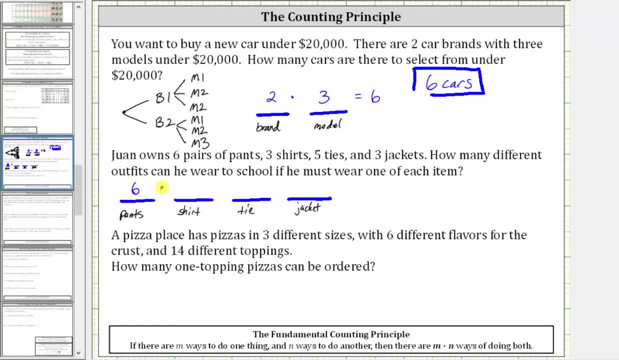 And since there are six pairs of pants, there are six ways to choose the pants times. since there are three shirts, there are three ways to choose the shirt times. since there are five ties, there are five ways to select the tie. 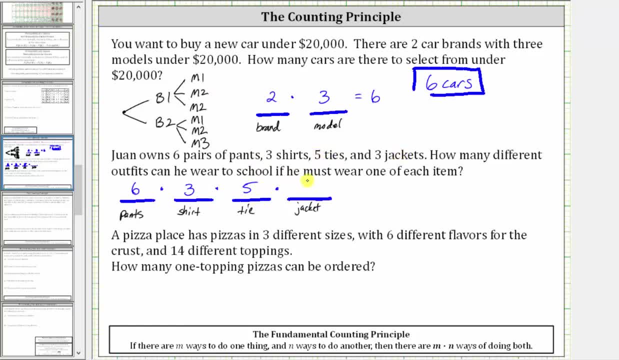 times. since there are three jackets, there are three ways to select the jacket. Six times three times five times three is equal to 270, which means there are 270 different outfits. Because there are so many outfits, you can see why we would not want to make a tree diagram.